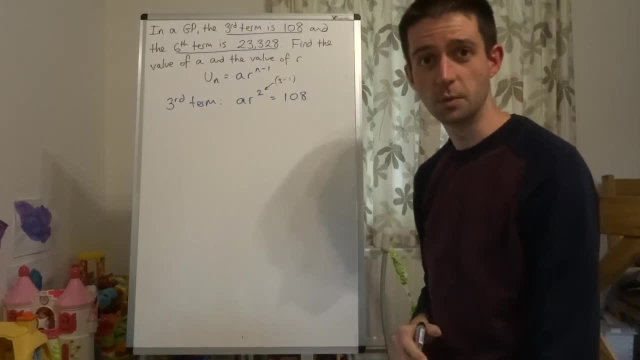 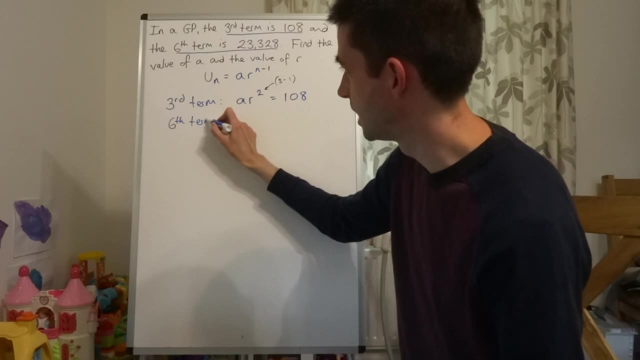 that's the number that I'm going to be using. So if I'm told that the third term is 108, two has come from three minus one. Similarly, I'm told the sixth term. So straight away I need to be really fluent by saying: right, sixth term, that's a r to the power of five, because the power is one. 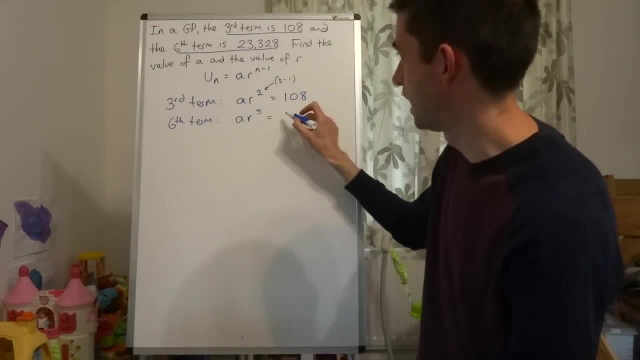 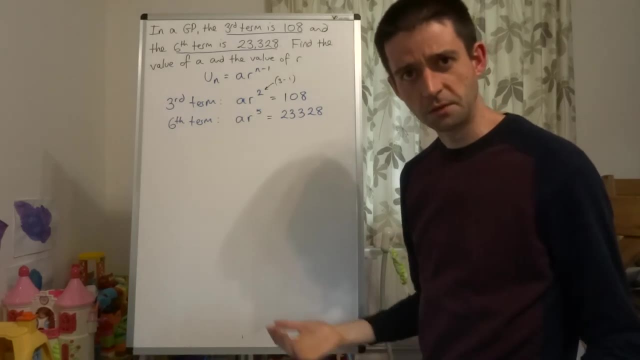 lower than the position. So a r to the power of five is 23,328.. So how do I use that to find a and r? Well, what I do is I'm going to be using a to the power of five. So if I'm told that the third term is r to the power of five. So I'm going to be using a and r squared. So I'm going to be using a to the power of five. So what I do is I'm going to be using a and n and r squared, And what I'm going? 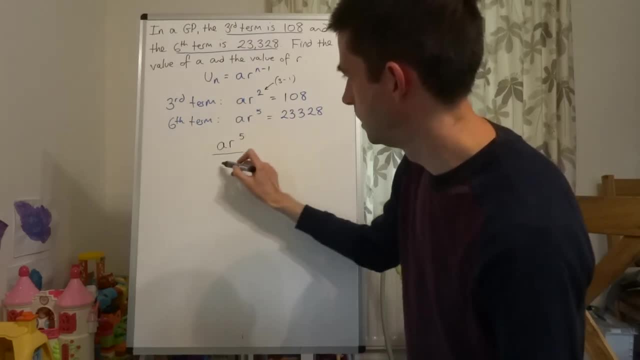 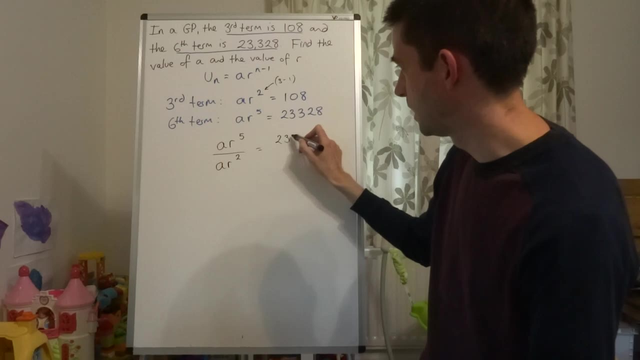 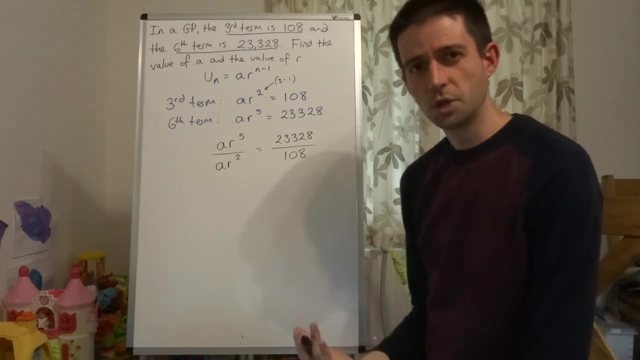 to do is I say that a r to the power of five divided by over a r squared, must be equal to 23,328 divided by 108.. And what's the point of doing that? Well, the point of doing that is on the 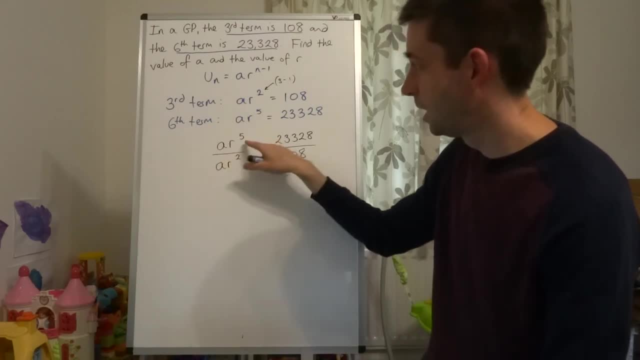 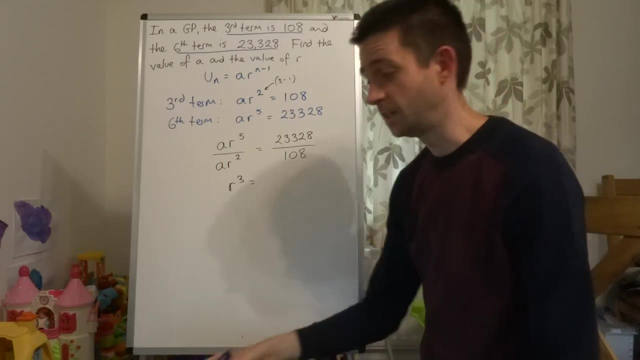 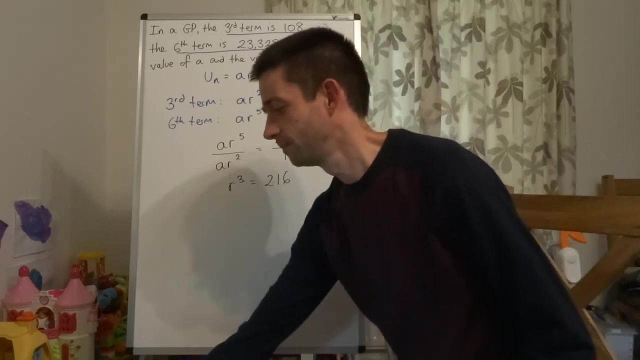 left-hand side: a divided by a cancels R to the five divided by r, squared is r cubed, because you subtracting the powers when you divide, And if I do 23,328 divided by 108, I'm hoping for a nice cube number as an answer which you do get is 260.. 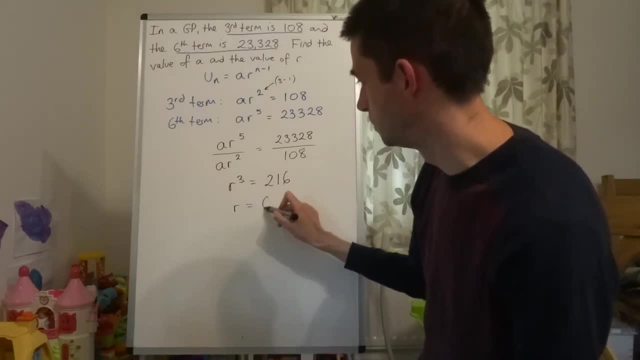 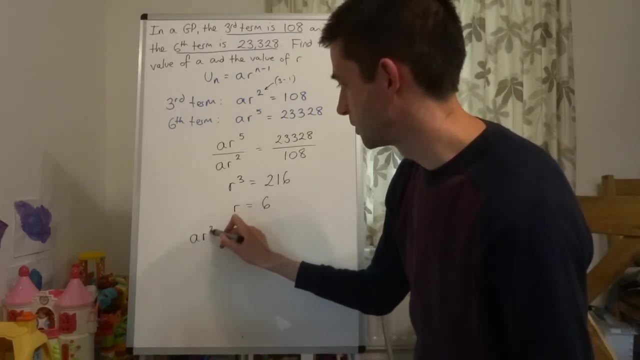 What that means is: if you take the cube root, then r must equal six. Don't forget to find a. We know that a r squared is 108.. That's using the third term. So a times by six squared is 108.. 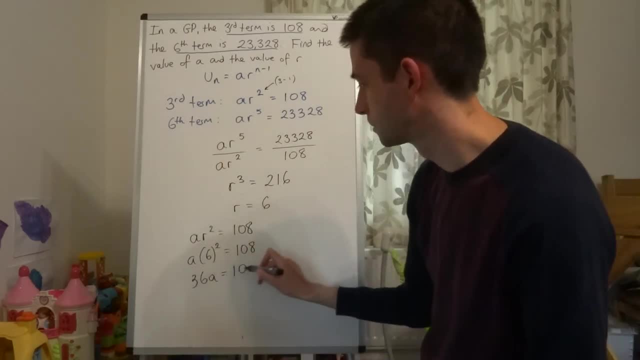 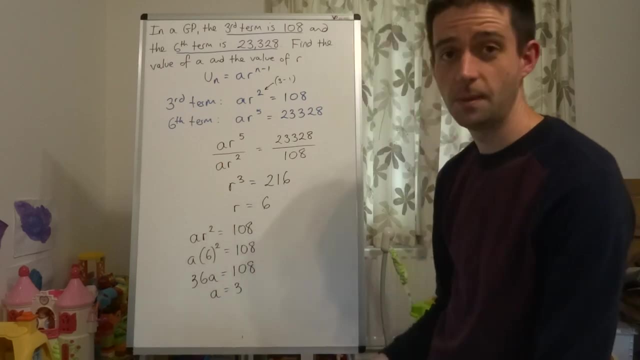 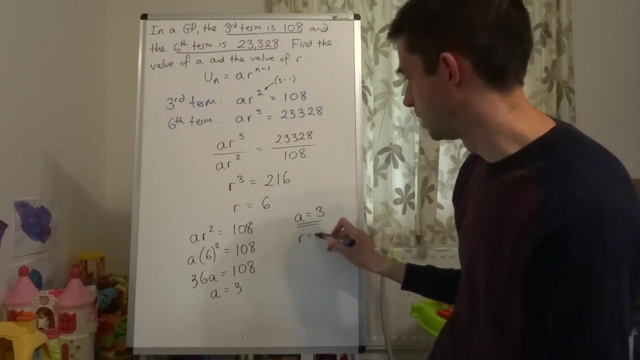 Six squared is 36,, which means that 36a is 108.. So dividing through, we have that a is three. So we have found that for this equation the sequence, the first term is three and the common ratio is six. 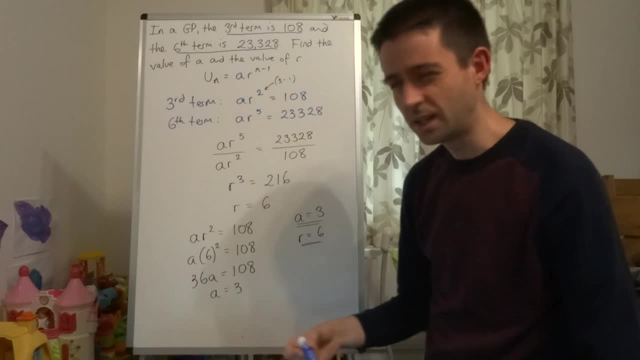 And if you really wanted to check, you could do it with this one. I wouldn't always advise it, but you could just check with this one. You could say: OK, well, if the first term is three and I'm multiplying by six, 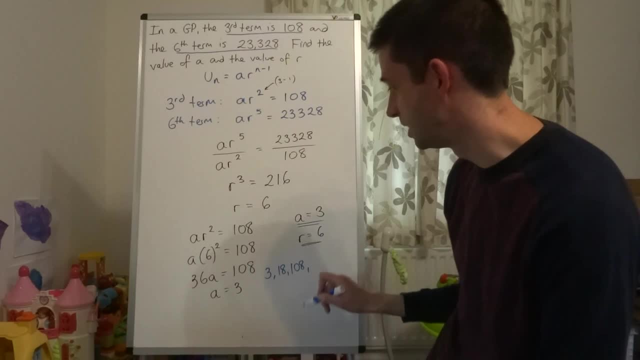 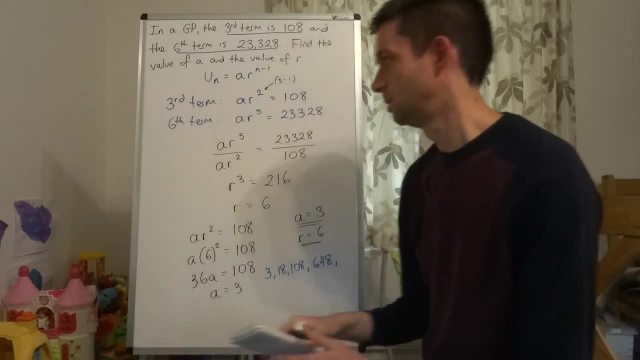 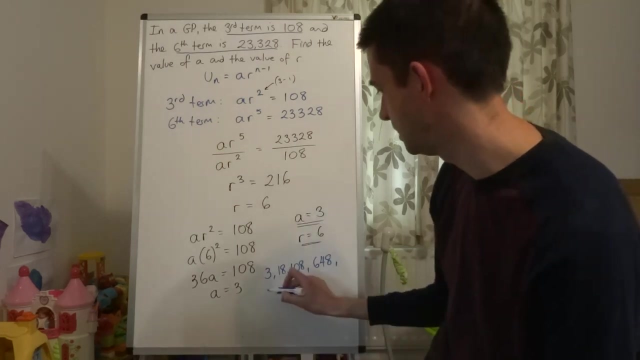 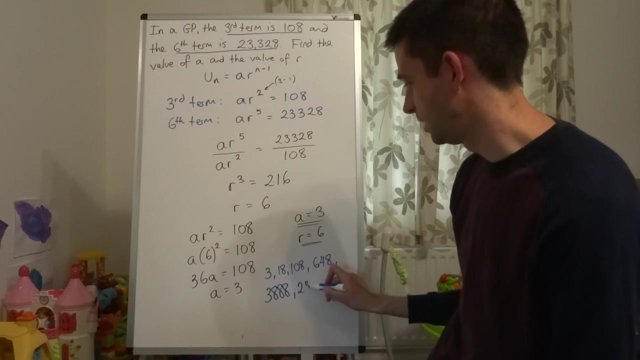 I'm going to get 18 times by six. One hundred and eight Happy days. Times by six. Six hundred and forty eight, Forty Six, four, eight times six, three, eight, eight, eight, And then times by six again, Twenty three thousand three hundred and twenty eight. 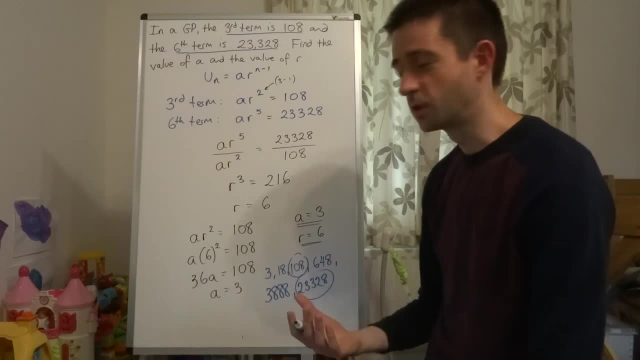 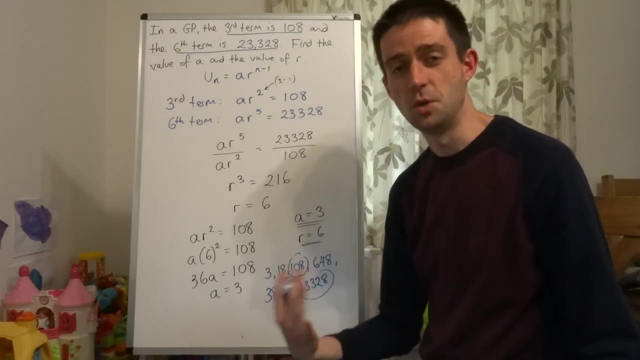 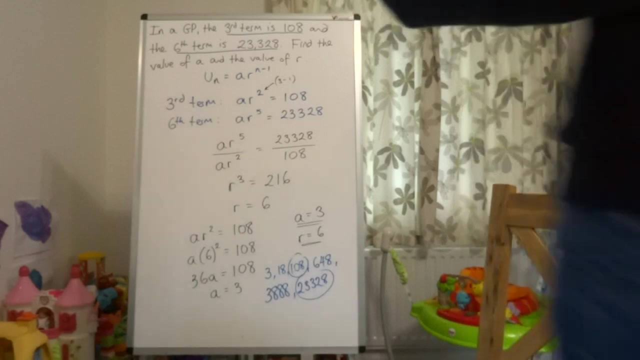 So there you go, Third term, sixth term, as required. A is three, R is six, And you could then be asked to do something subsequently with those values, because you now have everything you need to investigate the sequence further. Thank you. 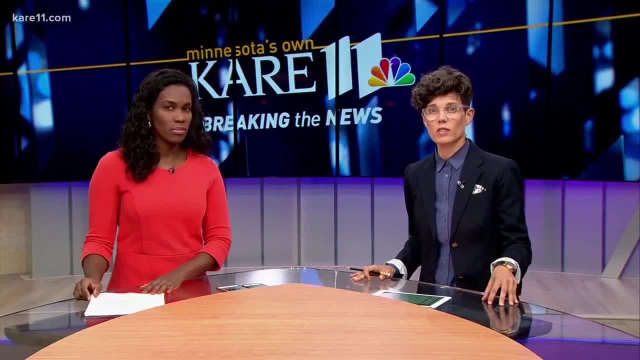 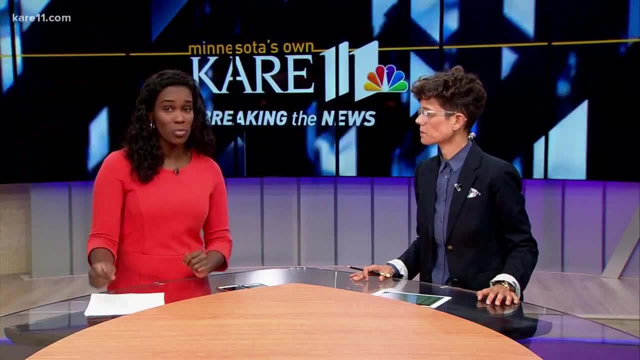 After 72 people were shot in one weekend in the city of Chicago, that city's mayor is calling for everyone there to work together. And Jenna, that violent weekend is also shining a spotlight on another issue, and it's an issue some don't talk about. 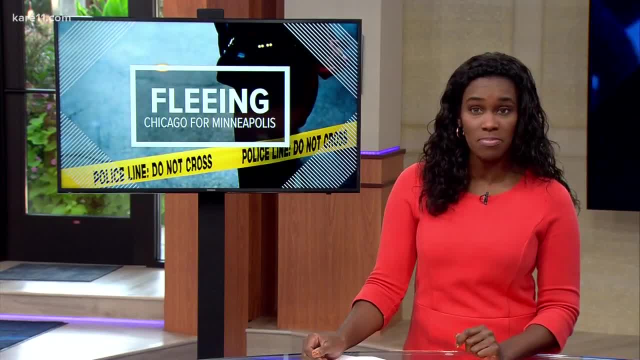 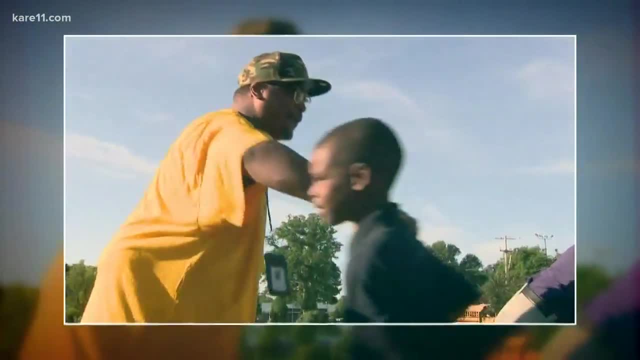 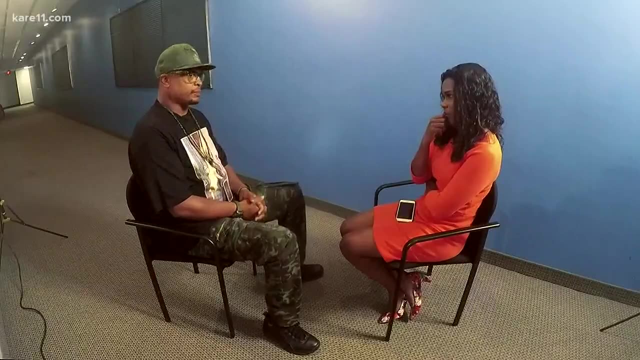 Who is killing these black victims? Not whites, not the police, but other blacks. Look at that smile. He ready for school. KG Wilson bears a heavy cross. literally, And this cross is about 400 pounds. And figuratively, Sometime I feel alone. Sometime I feel alone. 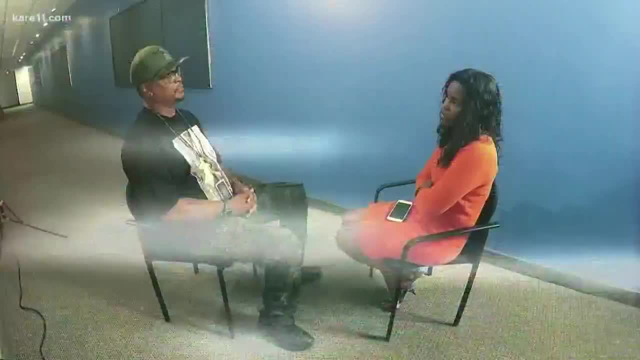 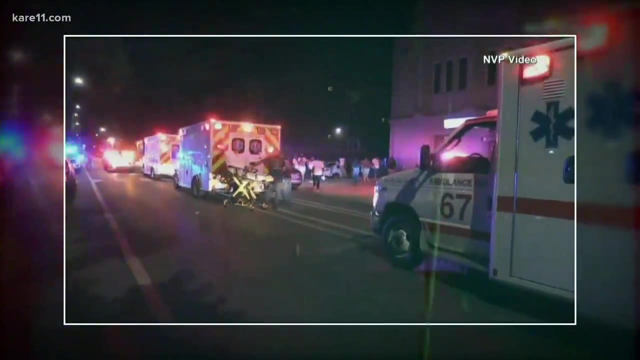 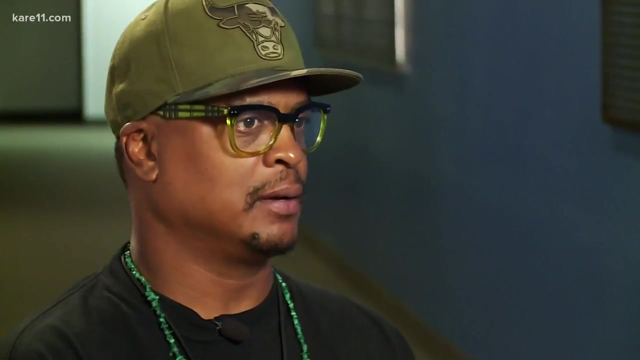 Alone, responding to a silent call for help. KG's past is embedded in Chicago's present. This weekend, 72 people were shot and at least 13 were killed. KG's heart is heavy. The violence here and the violence back home in Chicago. 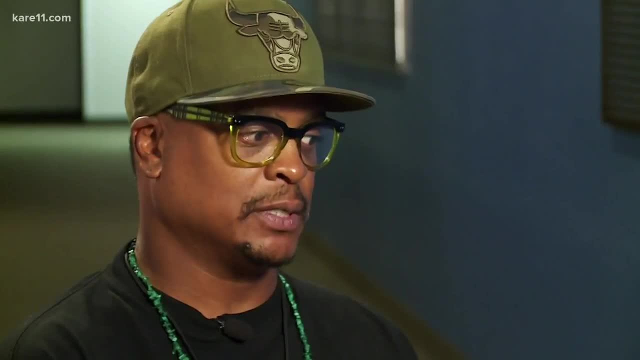 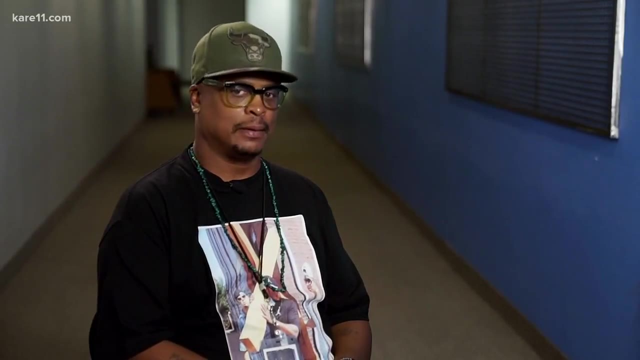 What my mission has been For 15 years now is the focus on us, And when I mean people of color. it's something that is kept a secret, And many times it's connected to stop snitching, Snitches, get stitches. 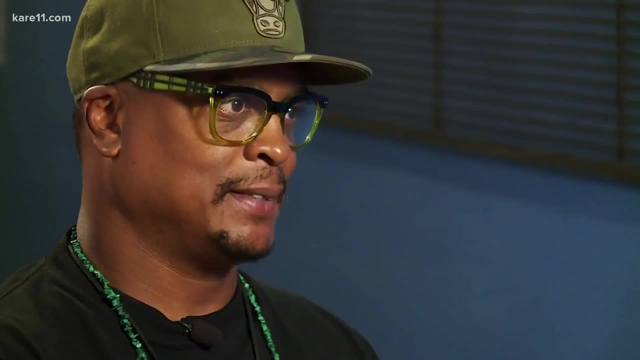 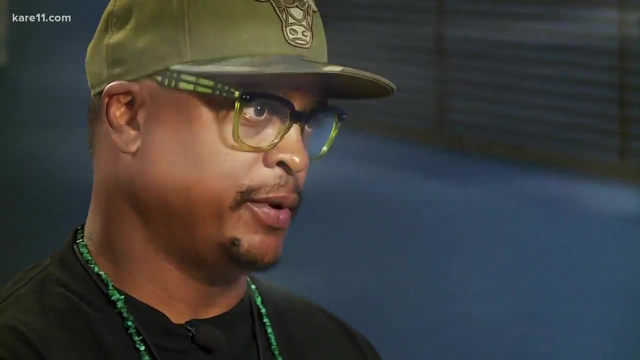 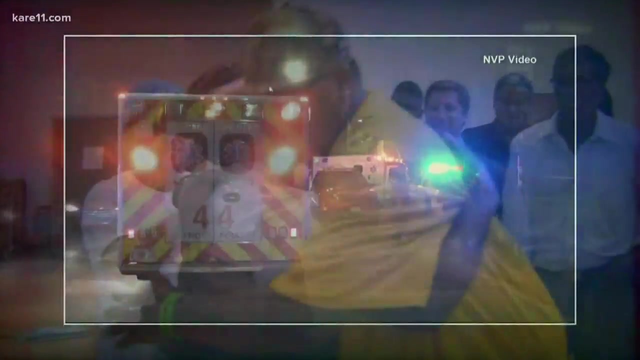 Yes, Yes. And the ones that don't get snitched on continue to hurt and kill and terrify and destroy our community. No arrests have been made in any of Chicago's weekend incidents incidents 15 years ago. Wilson and his son- now peace activists- escaped Chicago's violence.